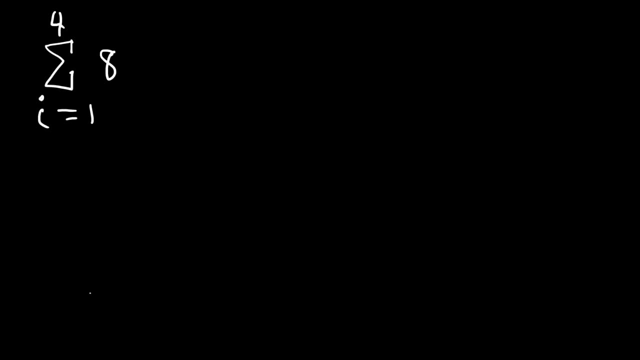 is this equal to? Now, there is a formula for this type of problem. If you have a constant c and if i is equal to 1 and it goes up to n, then it's going to equal the constant times n. In this case, we're adding 8 four times, so the constant is 8.. 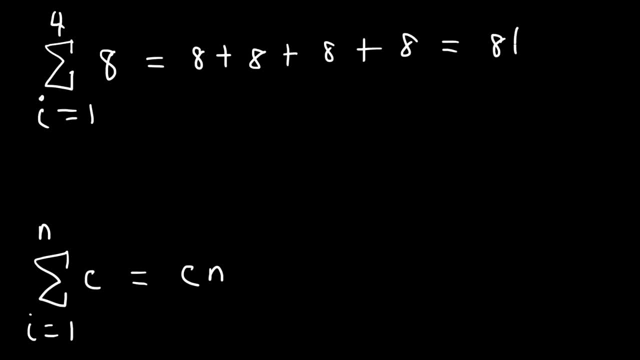 So, therefore, adding 8 four times is the same as multiplying 8 by 4, and this will give you 32.. Now let's work on some other examples. Try these two problems. Let's say i is 1,, the constant is 7 and this is 8, and also let's say this is 9 and this is 5.. 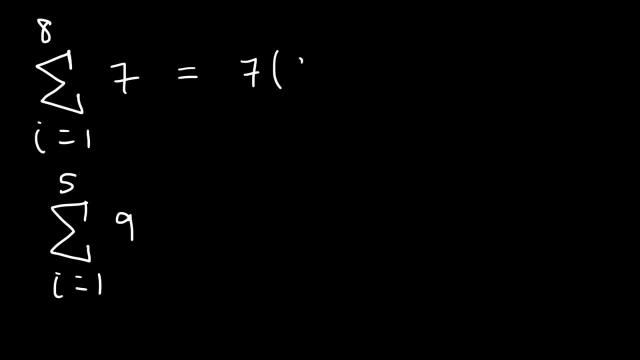 So the first one is simply going to be c times n, 7 times 8, so that's 56.. For the second example, it's going to be c times n, or 9 times 5, which is 45.. So that's how. 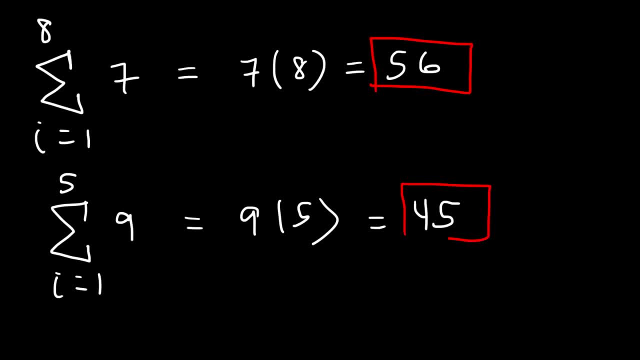 you can evaluate a sum if you have a constant. Now, the next formula that you need to be familiar with is this one. So, instead of a constant, we're going to have the variable i and we're going to go up to n. So this: 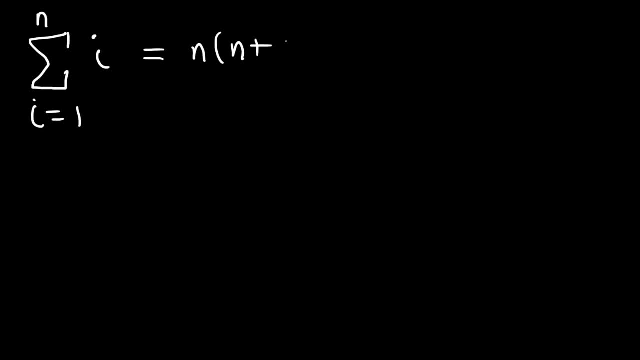 is going to equal n times n plus 1 divided by 2.. So let me give you an example. So let's say i is 1 and we have the variable i, And let's go up to 5.. So we need to add up all the numbers from 1 to 5.. 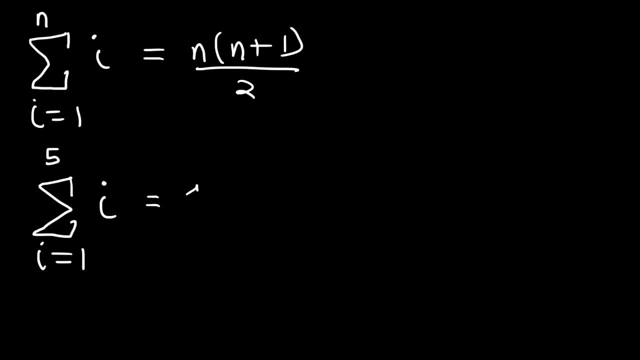 So when you replace I with 1,, you get 1.. If you replace it with 2, it's going to be 2.. And we're dealing with sums, so we have to add everything up to 5.. 1 plus 2 is 3.. 3 plus 3 is 6.. 6 plus 4 is 10.. 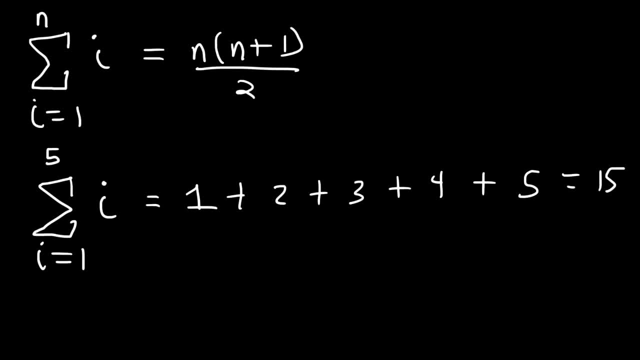 10 plus 5 is 15.. Now let's confirm that answer using the formula above. So n is this top number, It's 5.. So it's going to be 5 times 5 plus 1 divided by 2.. 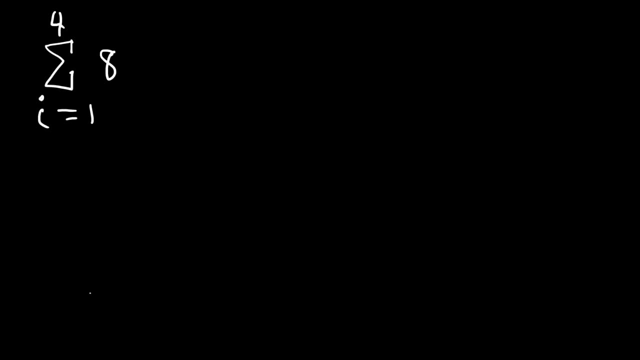 is this equal to? Now, there is a formula for this type of problem. If you have a constant c and if i is equal to 1 and it goes up to n, then it's going to equal the constant times n. In this case, we're adding 8 four times, so the constant is 8.. 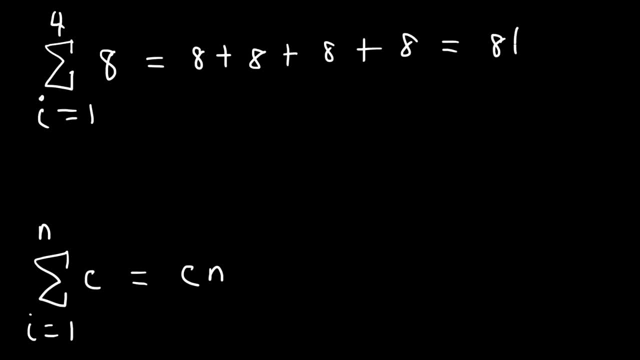 So, therefore, adding 8 four times is the same as multiplying 8 by 4, and this will give you 32.. Now let's work on some other examples. Try these two problems. Let's say i is 1,, the constant is 7 and this is 8, and also let's say this is 9 and this is 5.. 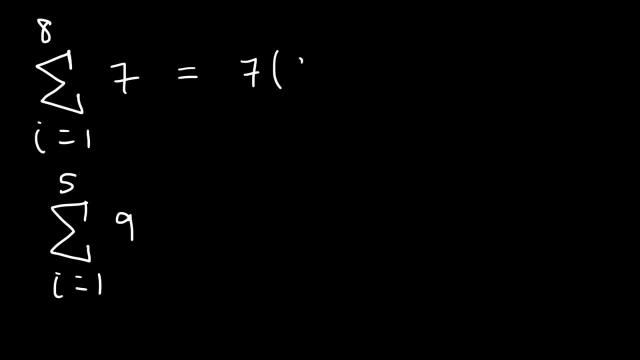 So the first one is simply going to be c times n, 7 times 8, so that's 56.. For the second example, it's going to be c times n, or 9 times 5, which is 45.. So that's how. 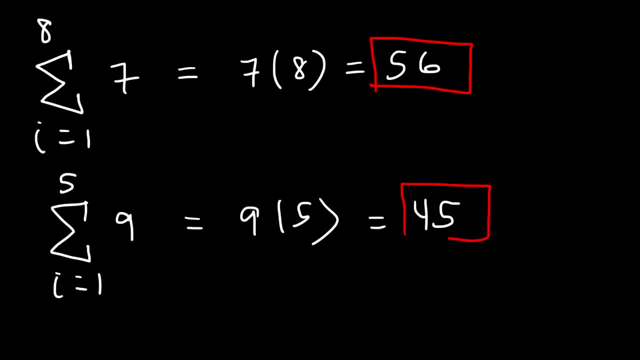 you can evaluate a sum if you have a constant. Now, the next formula that you need to be familiar with is this one. So, instead of a constant, we're going to have the variable i and we're going to go up to n. So this is going to equal n times n plus 1 divided by 2.. So let me give you an example. 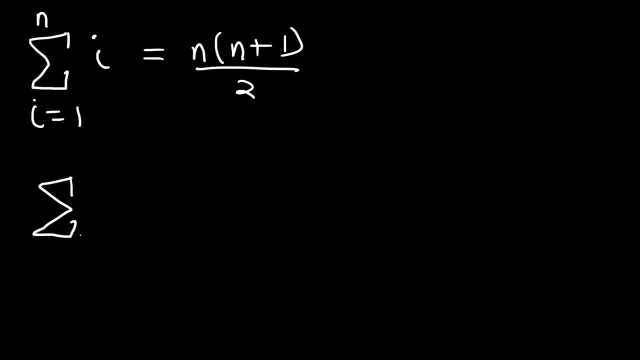 So let's say i is 1 and we have the variable i, And let's go up to 5. So we need to add up all the numbers from 1 to 5.. So when you replace i with 1, you get 1.. 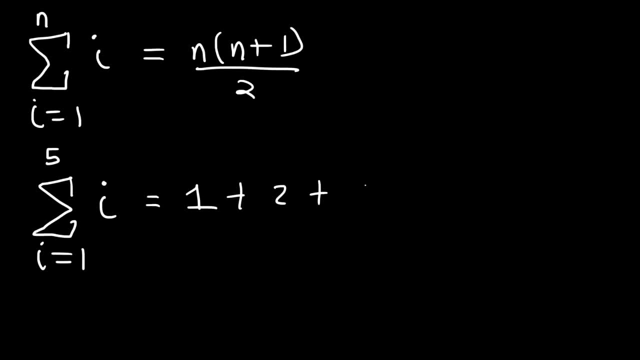 If you replace it with 2, it's going to be 2. And we're dealing with sums, so we have to add everything up to 5.. 1 plus 2 is 3.. 3 plus 3 is 6.. 6 plus 4 is 10.. 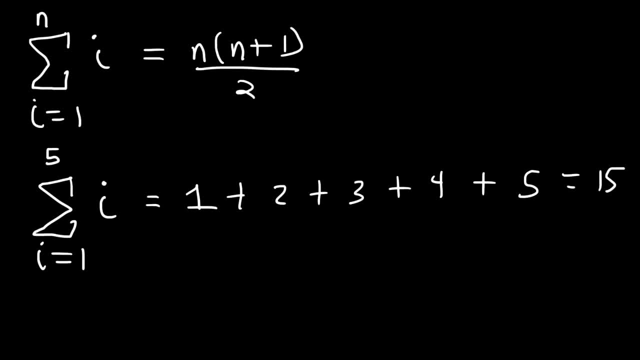 10 plus 5 is 15.. Now let's confirm that answer using the formula above. So n is this top number, It's 5.. So it's going to be 5 times 5 plus 1 divided by 2.. 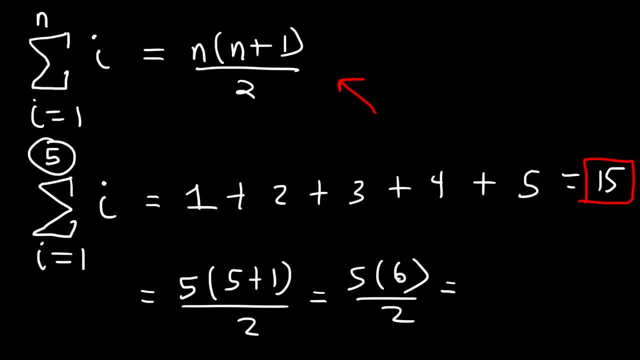 5 plus 1 is 6. And 6 divided by 2 is 3. And 5 times 3 is 15.. So, as you can see, this will give you the same answer. Try this problem. So let's say, if we have 6 times i, where i starts from 1 and it stops at 4.. 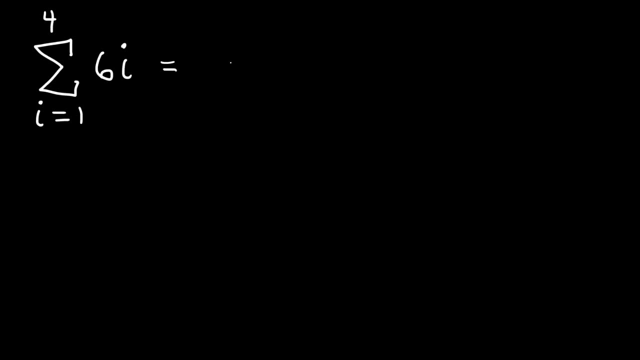 Go ahead and evaluate this sum. So when i is 1, 6 times 1 is 6.. When i is 2, 6 times 2 is 12.. 6 times 3 is 18.. 6 times 4 is 24.. 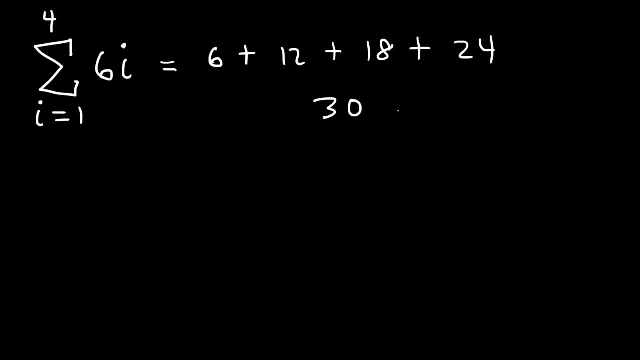 Now, 12 plus 18,, that's 30. And 6 plus 24 is also 30.. 30 plus 30 is 60. So that's the sum for this example. Now let's use the formula to confirm the answer. 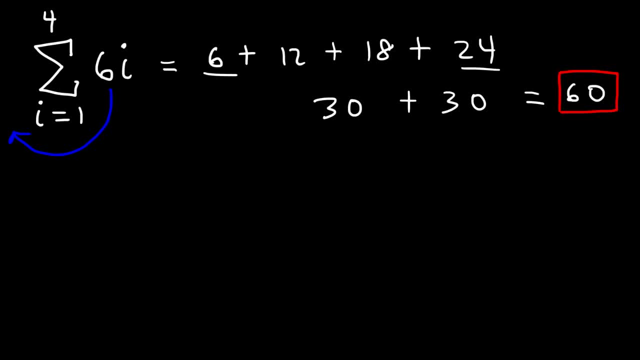 So what I'm going to do is take the constant and move it to the front. So what I have is 6 times the sum of i equals 1 to 4 for the variable i. So it's going to be 6 times n, n plus 1, divided by 2, where n is the top number 4.. 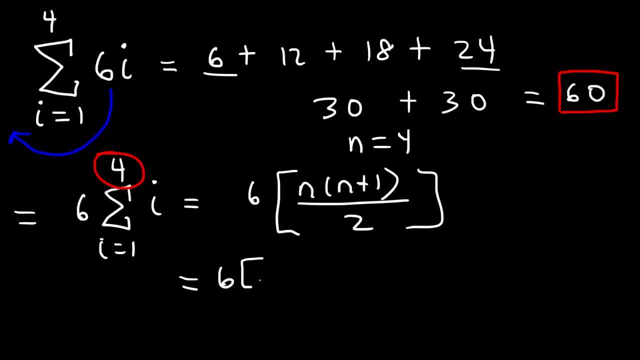 So that's going to be 6 times 4, and then 4 plus 1,, all divided by 2.. Now 4 divided by 2 is 2. And 4 plus 1 is 5.. 2 times 5 is 10, and 6 times 10 is 60. 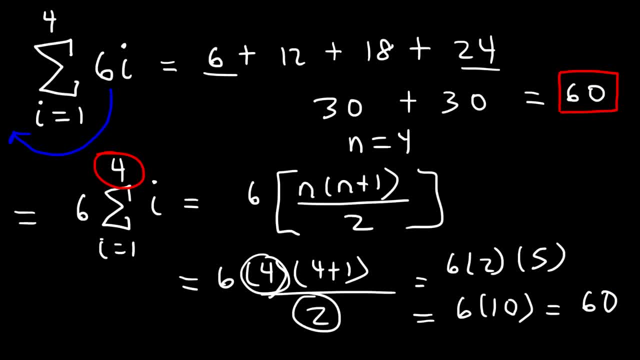 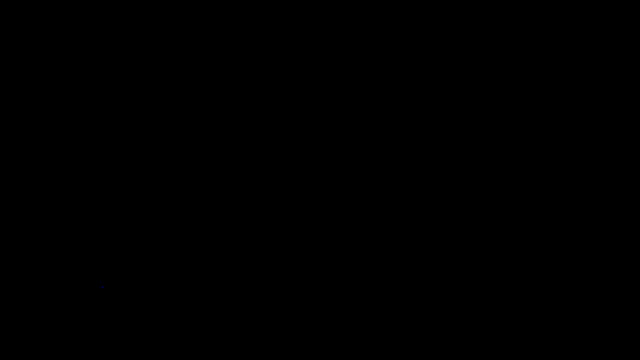 So in the end we get the same answer. So that's how you can use the formula to evaluate that particular sum. Let's try another example. Evaluate this one. So let's say, if this is 7i minus 3, going from 1 to 5.. 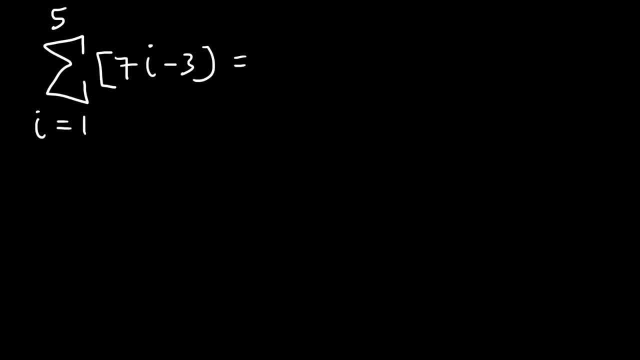 Go ahead and try that. So if we plug in 1, 7 times 1 minus 3 is 4.. If we plug in 2, 7 times 2 is 14, minus 3 is 11.. Good, 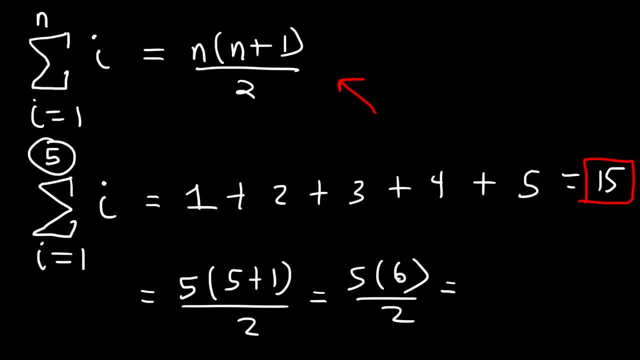 5 plus 1 is 6. And 6 divided by 2 is 3. And 5 times 3 is 15.. So, as you can see, this will give you the same answer. Try this problem. So let's say, if we have 6 times I, where I starts from 1 and it stops at 4.. 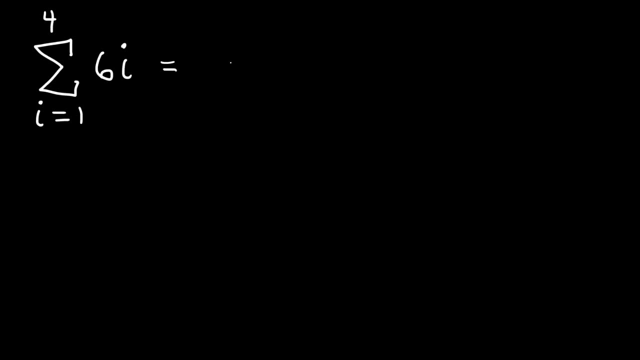 Go ahead and evaluate this sum. So when I is 1, 6 times 1 is 6.. When I is 2, 6 times 2 is 12.. 6 times 3 is 18.. 6 times 4 is 24.. 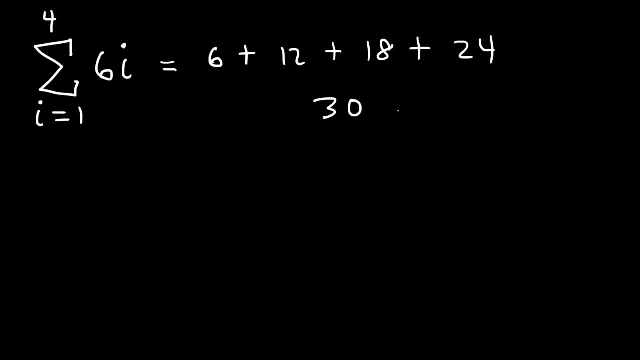 Now, 12 plus 18,, that's 30. And 6 plus 24 is also 30.. 30 plus 30 is 60. So that's the sum for this example. Now let's use the formula to confirm the answer. 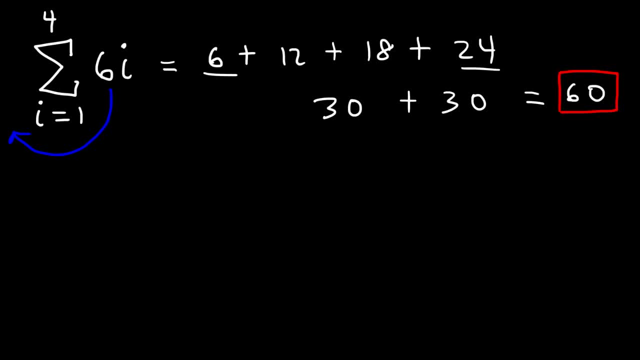 So what I'm going to do is take the constant and move it to the front. So what I have is 6 times the sum of I equals 1 to 4 for the variable I. So it's going to be 6 times n, n plus 1, divided by 2, where n is the top number 4.. 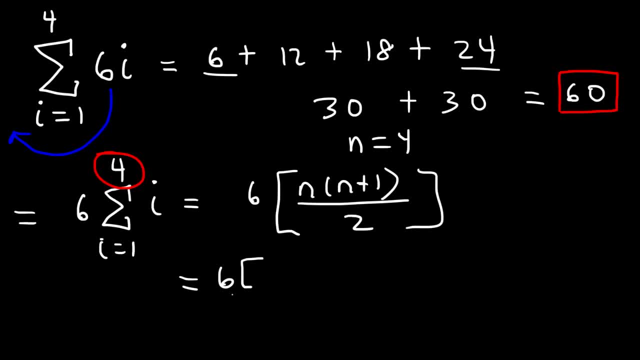 So that's going to be 6 times 4, and then 4 plus 1,, all divided by 2.. Now 4 divided by 2 is 2. And 4 plus 1 is 5.. 2 times 5 is 10, and 6 times 10 is 60. 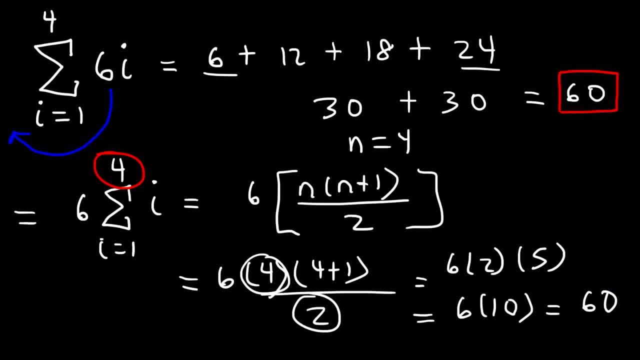 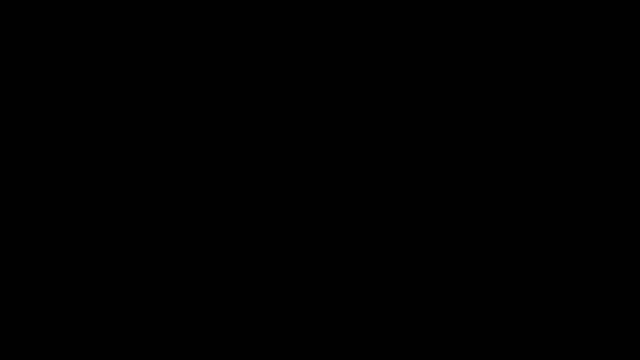 So in the end we get the same answer. So that's how you can use the formula to evaluate that particular sum. Let's try another example. Evaluate this one. So let's say, if this is 7i minus 3, going from 1 to 5.. 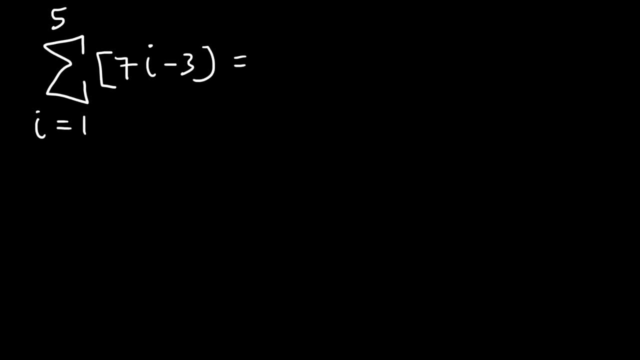 Go ahead and try that. So if we plug in 1, 7 times 1 minus 3 is 4.. If we plug in 2, 7 times 2 is 14, minus 3 is 11.. If we plug in 3, 7 times 2 is 12.. 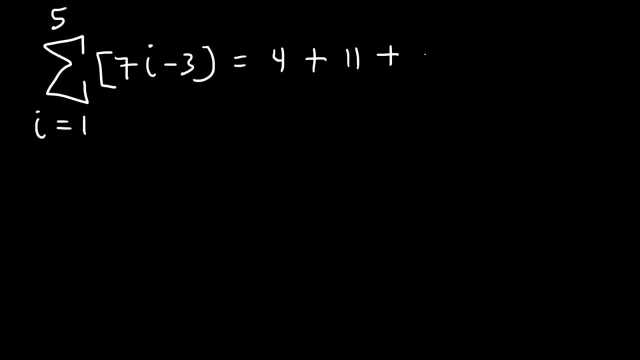 3,. 7 times 3 is 21,. minus 3 is 18.. Notice that the numbers are increasing by 7.. We have an arithmetic sequence, but with a sum. So the next number is going to be 25, and the 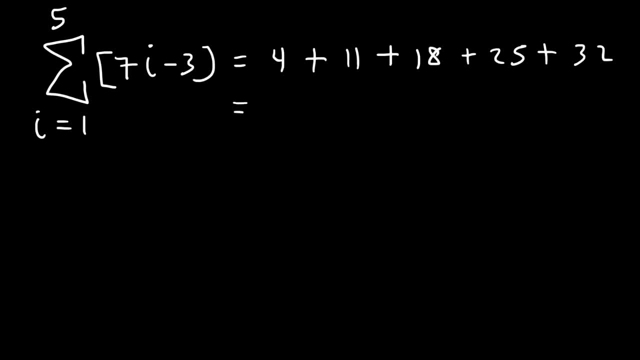 fifth one. the last one is 32.. Now, 4 plus 11 is 15.. And then, if we add 18 and 32, that's going to be 50. And then 15 and 25, that's 40. 40 plus 50 is 90. So the sum is 90. Now, 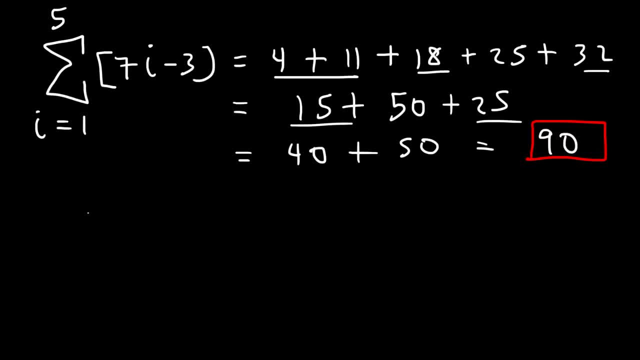 let's use the summation formulas to get the same answer. So I'm going to write it as 7 times the sigma notation for i, going from 1 to 5. And then minus 3.. We're going to separate it into two parts, So for i the formula is going to be: 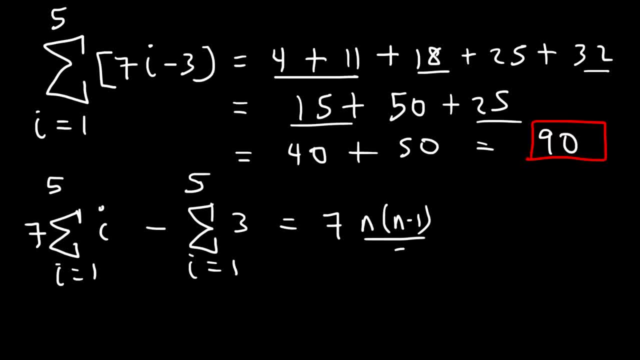 n times n minus 1, divided by 2.. And for the constant it's simply c times n, and the constant is 3, so it's going to be 3 times n, where n is 5.. So that's going to be 7 times 5, and 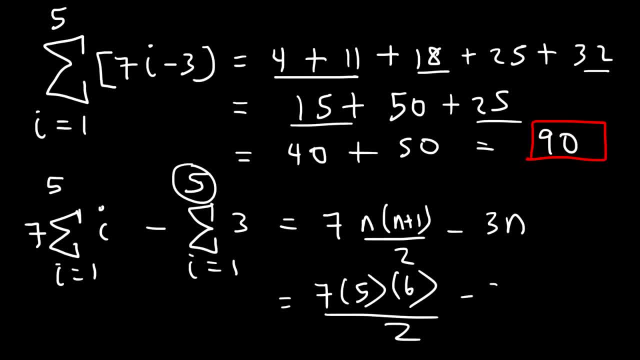 1 is 6.. And then this is going to be 3 times 5.. Now I'm running out of space so I'm just going to continue here. So I'm going to continue here. 7 times 5 is 35, and 6 divided by 2 is 3.. 3 times 5 is 15.. Now 35 times 3.. 30 times 3 is 90.. 5 times 3 is 15, so 90 plus 15.. 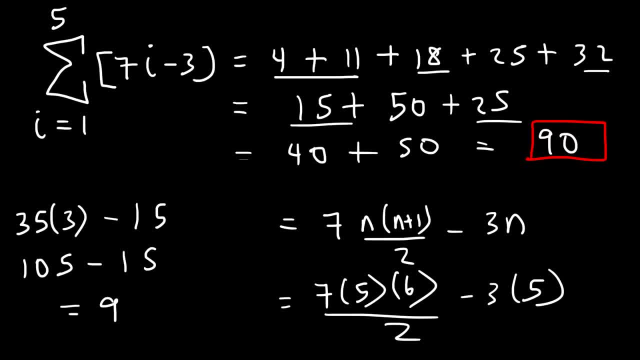 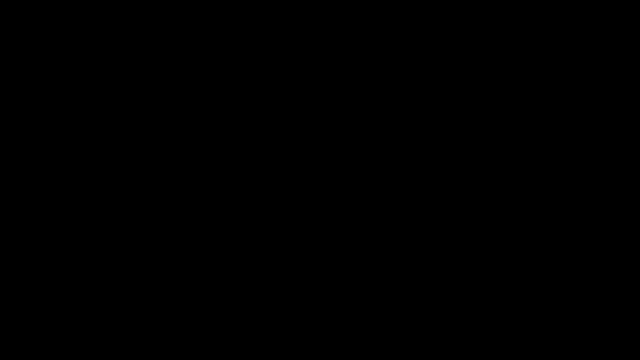 That's 1.. 105, and 105 minus 15 is 90, and so you get the same answer. now, for the sake of practice, go ahead and try in this example. feel free to pause the video if you want to try. let's say this is going to be 9i plus 7, so this is going to be. 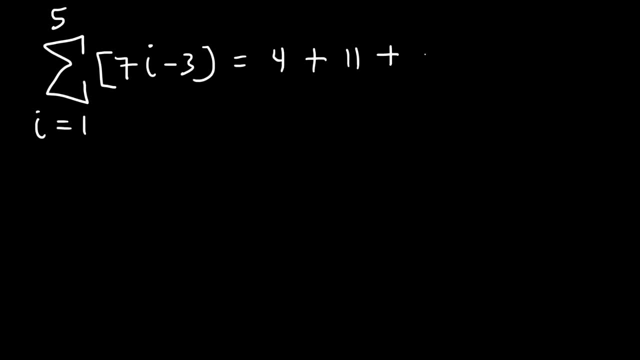 3.. 7 times 3 is 21.. Minus 3 is 18.. Notice that the numbers are increasing by 7.. We have an arithmetic sequence, but with a sum, So the next number is going to be 25.. And the 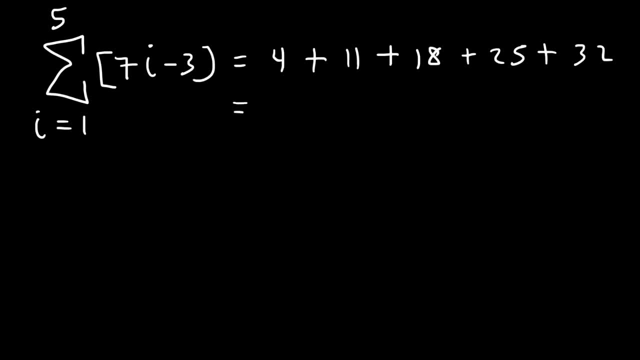 fifth one. the last one is 32.. Now, 4 plus 11 is 15.. And then, if we add 18 and 32, that's going to be 50. And then 15 and 25, that's 40. 40 plus 50 is 90. So the sum is 90. Now, 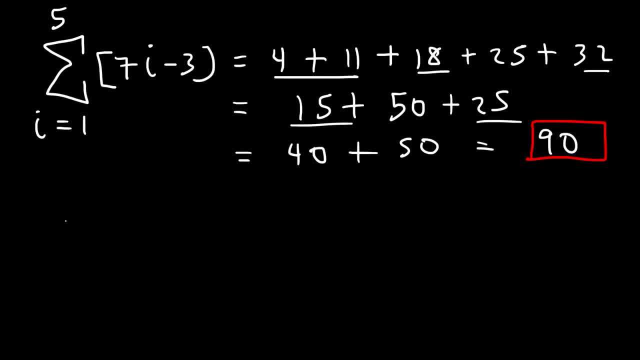 let's use the summation formulas to get the same answer. So I'm going to write it as 7 times the sigma notation for i, going from 1 to 5. And then minus 3.. We're going to separate it into two parts, So for i the formula is going to be n. 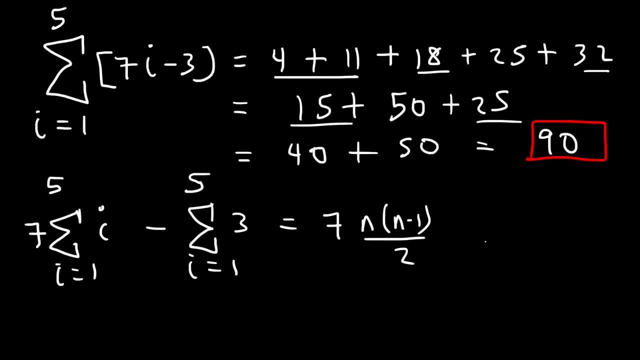 times n minus 1 divided by 2.. And for the constant it's simply c times n, And the constant is 3, so it's going to be 3 times n, where n is 5.. So that's going to be 7 times 5,. 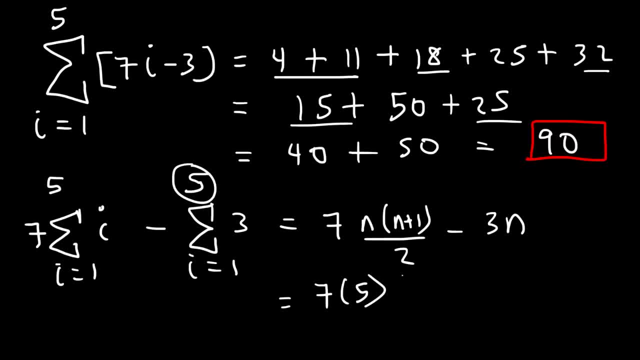 and it's supposed to be plus 1,, not minus 1.. 5 plus 1 is 6, and then this is going to be 3 times 5.. Now I'm running out of space, so I'm just going to continue here 7 times. 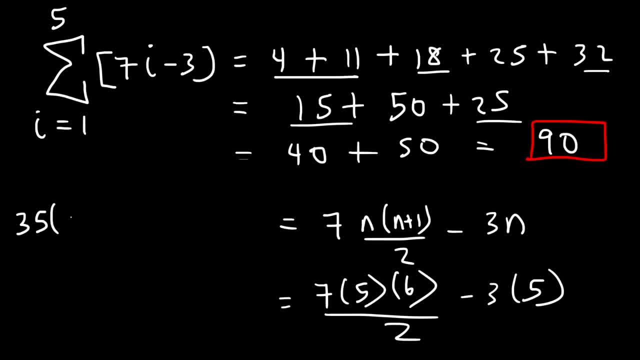 5 is 35, and 6 divided by 2 is 3.. 3 times 5 is 15.. Now, 35 times 3,, 30 times 3 is 90,. 5 times 3 is 90.. 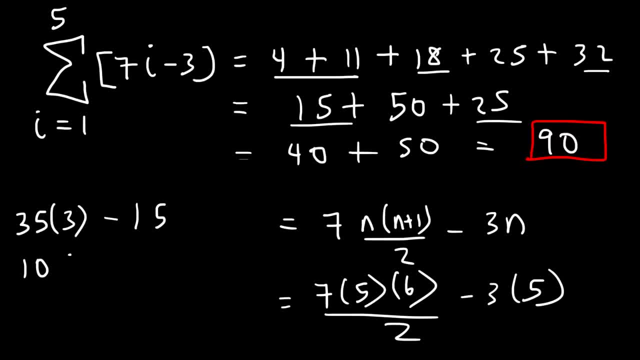 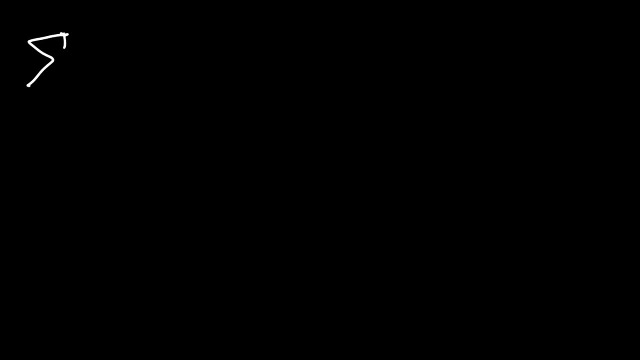 5 times 3 is 15, so 90 plus 15, that's 105.. And 105 minus 15 is 90. And so you get the same answer. Now, for the sake of practice, go ahead and try this example. Feel free to. 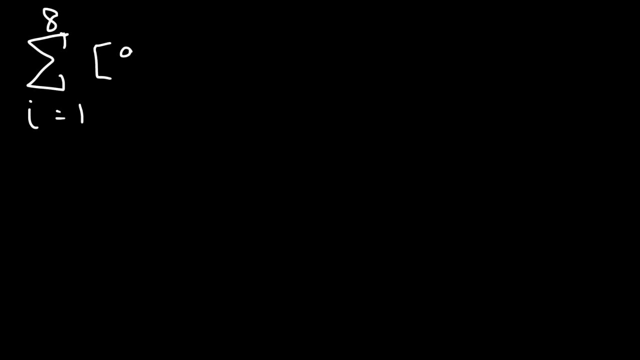 pause the video if you want to try it. Let's say: this is going to be 9i plus 7.. So this is going to be 9i plus 7.. So this is going to be 9i plus 7.. So this is going to be 9i. 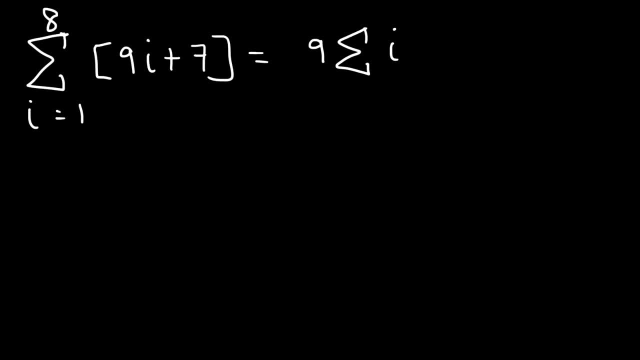 nine times the Sigma notation for I, going from 1 to 5, and plus the Sigma notation for 7 as a constant actually supposed to be 8 not 5, so n is 8. in this example, this is going to be 9 times n times n plus 1, divided by 2 plus 7 times. 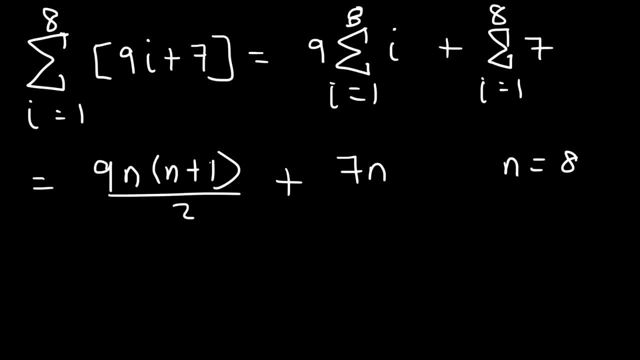 n where n is 8, so this is going to be 9 times 8. 8 plus 1 is 9 divided by 2, and then plus 7 times 8. now 9 times 9 is 81, and 8 divided by 2 is 4 and 7 times 8, 56, 81 times 4, 80 times. 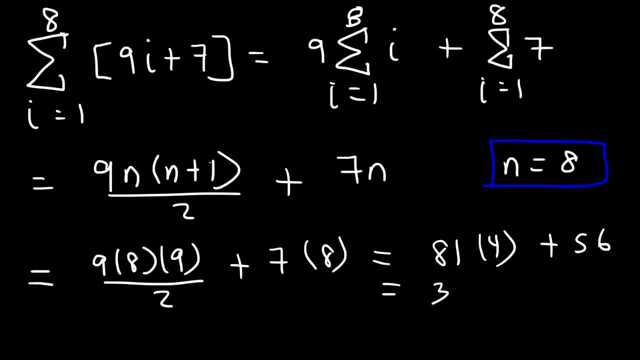 4 is 320, and then 1 times 4 is 4, so that's 324. if you add 56 to it, that's going to give you 380, which is the final answer. now let's confirm it using simple addition. so if we plug in one nine times one plus, 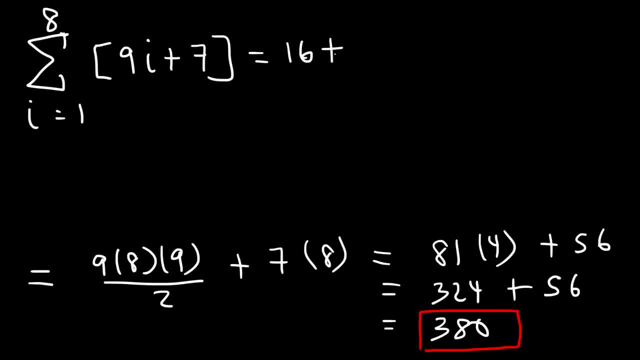 7, that's 16. and then, if we plug in two nine times two, is 18 plus 7, that's 25. and then three nine times three is 27 plus 7, 34, so it's going up by nine. the next one's going to be 43, that's the fourth number, and then 52, and then 61. 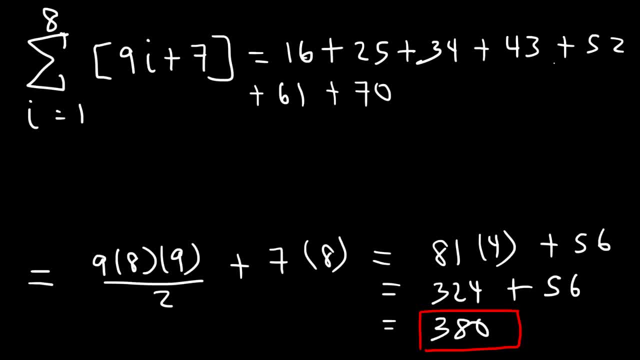 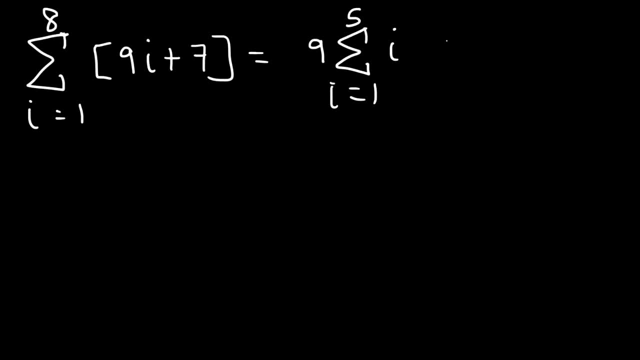 the sigma notation for i going from 1 to 5, and plus the sigma notation for 7 as a constant. Actually it's supposed to be 8, not 5.. So n is 8 in this example. This is: 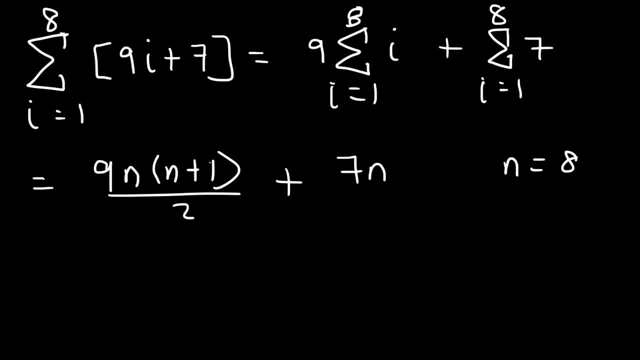 where n is 8. so this is going to be 9 times 8. 8 plus 1 is 9 divided by 2, and then plus 7 times 8. now 9 times 9 is 81, and 8 divided by 2 is 4, and 7 times 8 is 56. 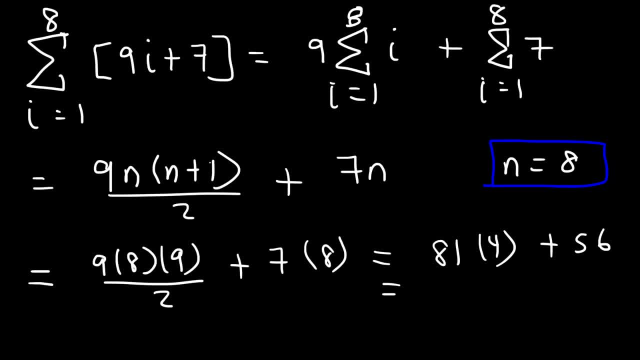 81 times 4, 80 times 4 is 320, and then 1 times 4 is 4, so that's 324. if you add 56 to it, that's going to give you 380, which is the final answer. now let's confirm it using simple addition. 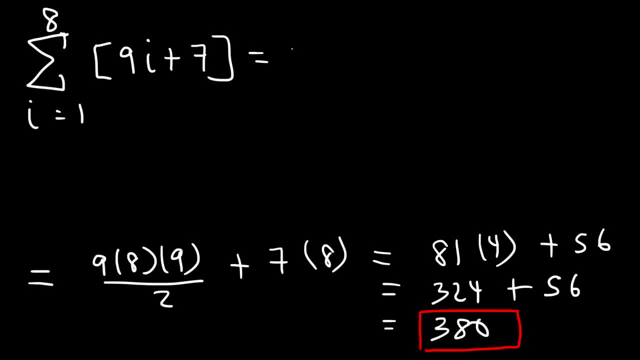 so if we plug in 1, 9 times 1 plus 7, that's 16, and then, if we plug in 2, 9 times 2 is 18 plus 7, that's 25, and then 3, 9 times 3 is 27 plus 7, 34, so it's going up by 9. the next one is going to be 43. that's the fourth number. 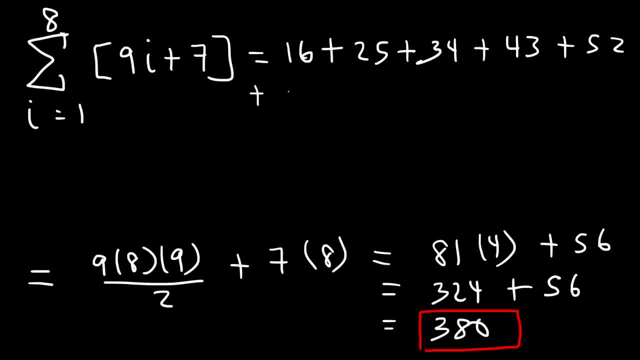 and then 52, and then 61, and then 70, so we have 7 numbers. now the last one is going to be 9 times 1 plus 7, that's 16. and then, if we plug in 2, 9 times 2 is 18 plus 7, that's 25. 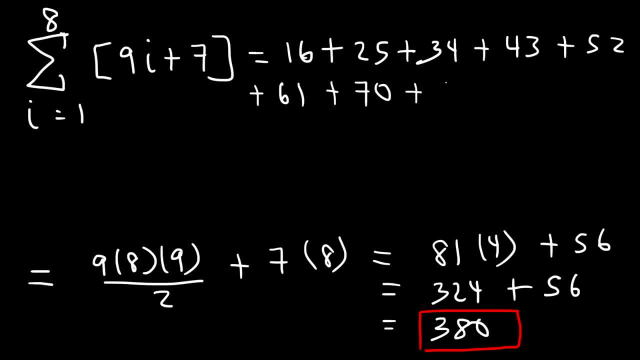 1, 9 times 8 is 72 plus 7, 79. so let's use a calculator for this. so if we add 16, 25, 34, 43, 52, 61, 70 and 77- I mean that's 77 but 79- this will give us 380, so we get the exact same answer. 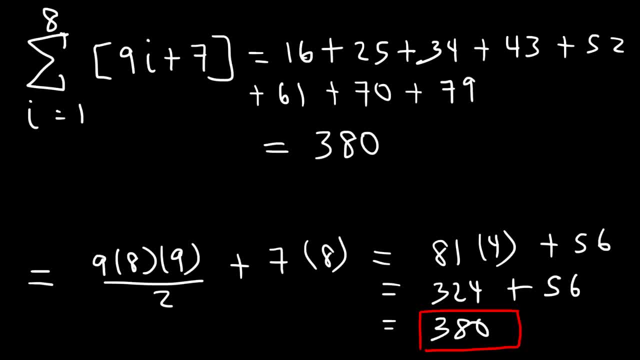 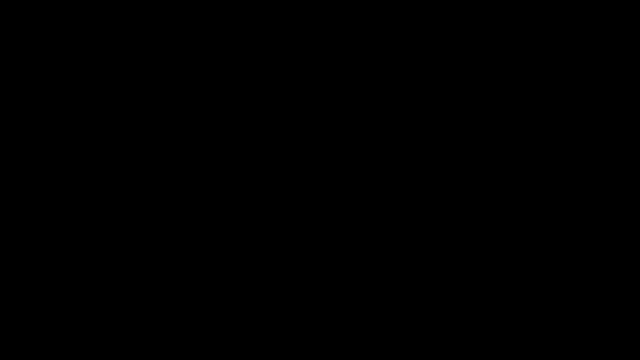 this will give us 380, so we get the exact same answer. now let's move on to the next version of this math test, next one, and it's this time I squared instead of I. it's equal to n times n plus 1 times 2n plus 1 divided by 6. so let's confirm that with an example. so 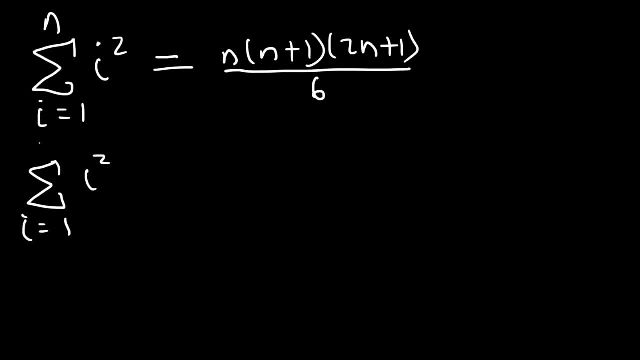 let's say, if we have I squared and we wish to go up to 6, this is going to be 1 squared plus 2 squared plus 3 squared plus 4 squared plus 5 squared plus 6 squared. so 1 squared is 1, 2 squared is 4, 3 squared is 9, 4 squared is 16, 5 squared. 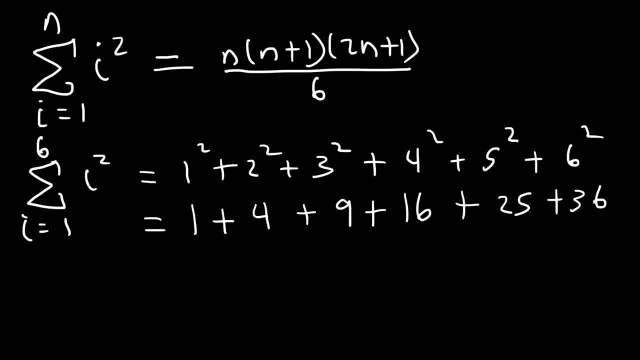 is 25, 6 squared is 36. now, if we add 1 plus 9, that's going to give us 10, and then if we add 4 and 16, that's going to give us a nice number. that's 20 and 25 and 36, 20. 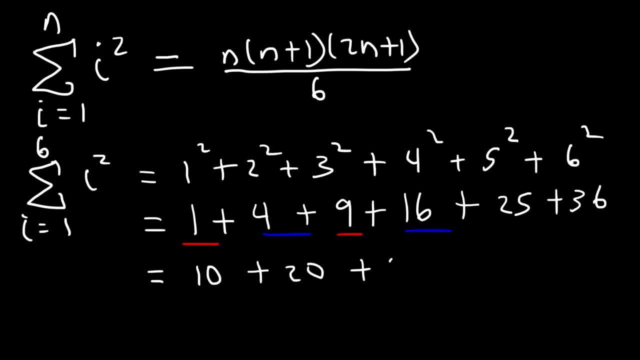 and 30 is 50. 5 and 6 11, that's going to be 61. 10 plus 20 is 30 plus 61, that's 91. now let's get the same answer using that formula. so let's erase this. so n is 6. 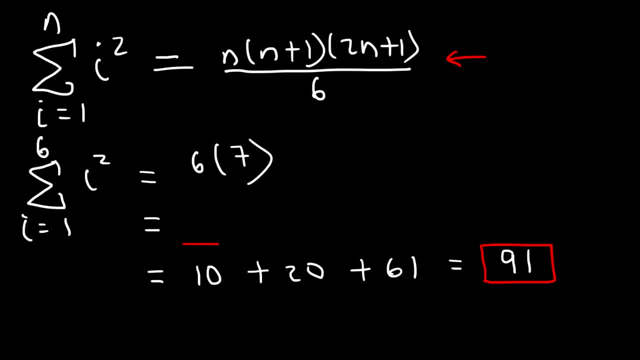 n plus 1, that's going to be 7, and then 2n plus 1, 2 times 6 is 12 plus 1, that's 13 divided by six. so we can cancel six. and then 7 times 13, 10 is 70, 7 times 3 is 21, 70 and 21 gives us 91. so this example confirms this. 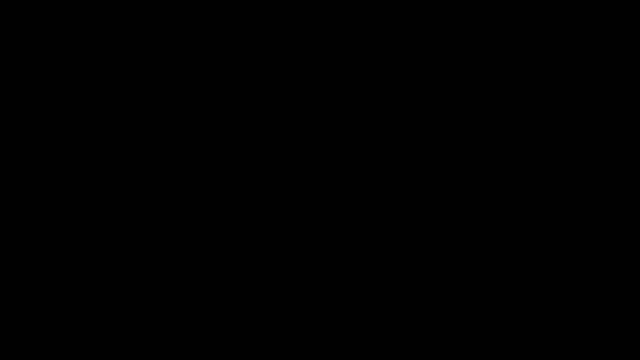 now let's move on to the next formula, and it's this time I squared instead of I. it's equal to n times n plus 1 times 2 n plus 1 divided by 6. so let's confirm that with an example. so let's say: if we have I squared and we wish to go up to 6, this is going to be 1 squared plus 2 squared plus 3 squared plus 4 squared plus 5 squared plus 6. 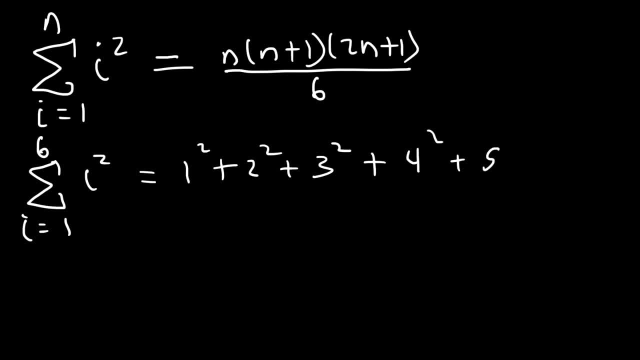 squared. so 1 squared is 1, 2 squared is 4, 3 squared is 9, 4 squared is 16 and 5 squared is 13, that's 65. so each of these are equation as usual. so that's the answer. so we publish that shape. 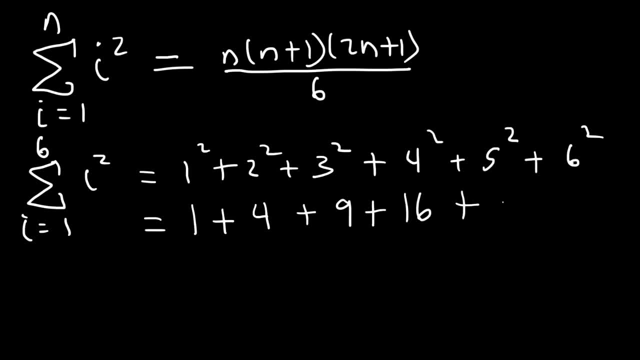 and we convert it into our real private number. that one time comes down here. so that's it: 5 squared is 25, 6 squared is 36. now, if we add 1 plus 9, that's going to give us 10. and then if we add 4 and 16, that's going to give us a nice number, that's 20. 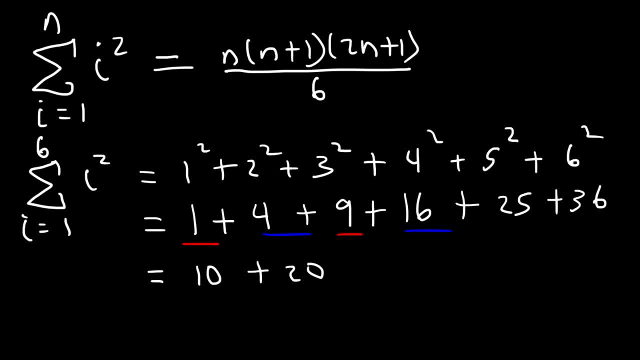 and 25 and 36, 20 and 30 is 50, 5 and 6: 11, so that's going to be 61. 10 plus 20 is 30 plus 61, that's 91. now let's get the same answer using that formula. so let's. 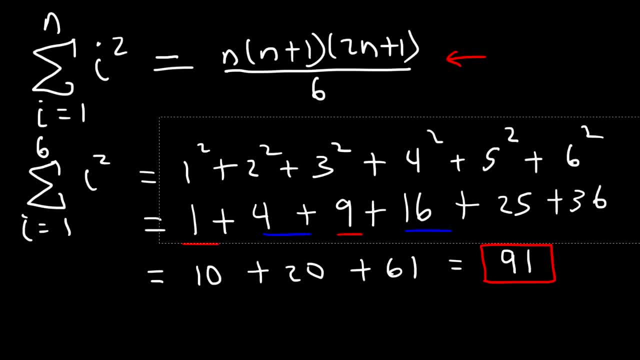 erase this. so n is 6 and plus 1, that's going to be 7, and then 2n plus 1. 2 times 6 is 12 plus 1, that's 13 divided by 6. so we could cancel 6 and then 7 times 13, 7 times 10 is 70, 7 times 3 is 21, 70 and 21. 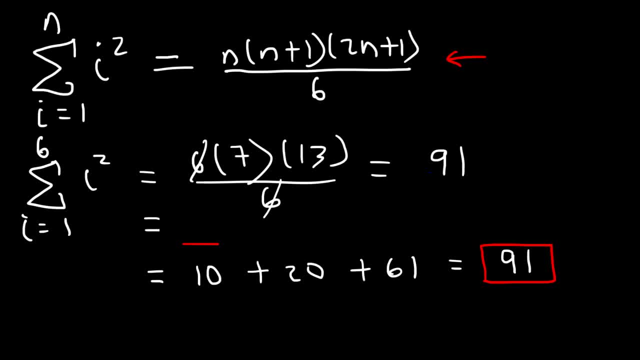 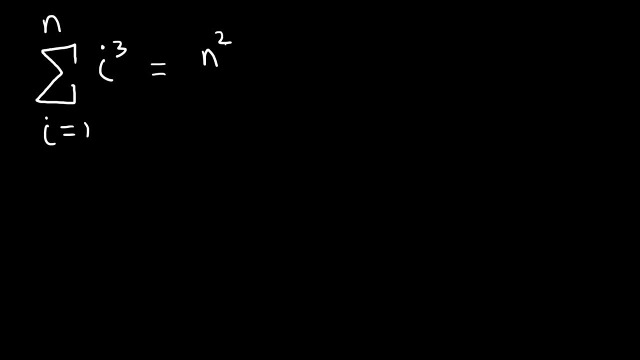 gives us 91. so this example confirms this formula. now the last formula that we need to talk about is i to the third power. so it's going to be n squared times n plus 1 squared divided by 4. so let's use an example. let's say n is 4, let's keep it simple. so this is going to be one to. 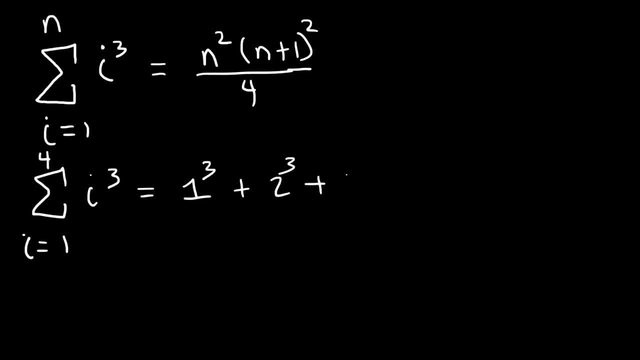 the third, plus two to the third, plus three to the third, plus four to the third power. so 2 to the third is 8, 3 cube is 27, 4 cube is 64. so 1 plus 8 plus 27 plus 64, that's equal. 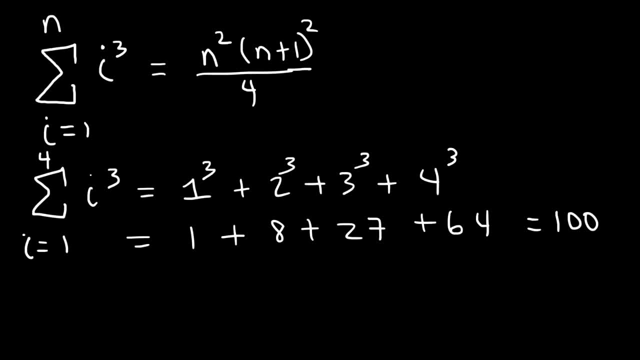 to 100. now let's see if we can get the same answer using this formula. so i'm going to work it right here. so n is 4, that's going to be 4 squared, and 4 plus 1 is 5 and 4 plus. 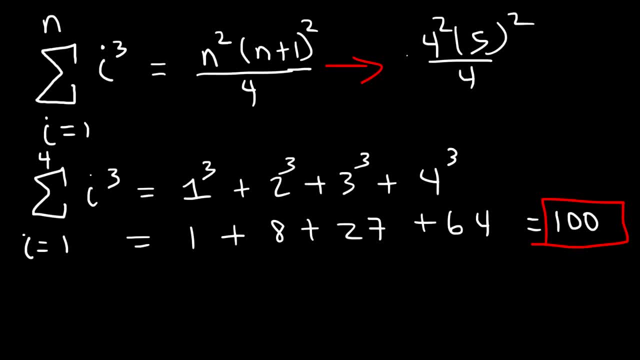 1 is 5 divided by 4, so we can cancel a 4, leaving one 4 on top. 5 squared is 25, and 4 times 25 is 100. so this is the formula for i to the third. if you ever need to use it now, let's. 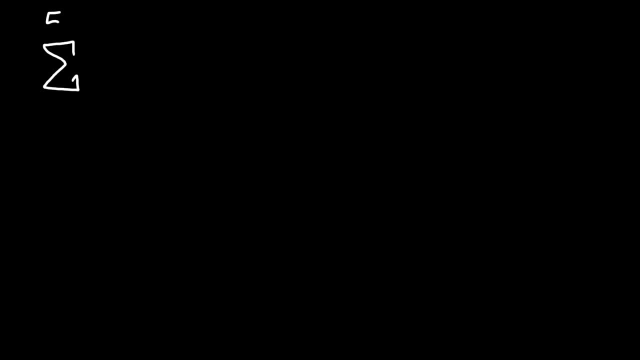 work on a few practice examples. so let's say, if we have i times i squared plus 4, i go ahead and try this now. the first thing i recommend doing is to distribute the i to i squared plus 4i. so this is going to be i to the third power, and then i times 4i, that's. 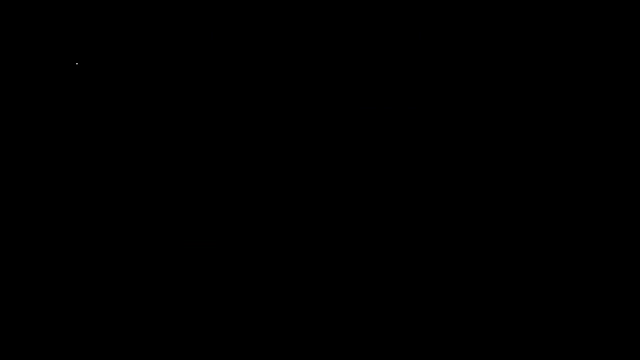 formula. now, the last formula that we need to talk about is I to the third power. so it's gonna be n squared times n plus 1 squared divided by 4. so let's use an example. let's say n is 4, let's keep it simple. so this is going to be 1 to 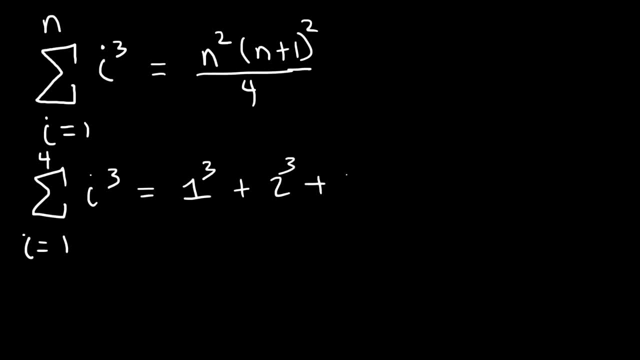 the third plus 2 to the third, plus 3 to the third plus 4 to the third power. so 2 to the third is 8, 3 cube is 27, 4 cube is 64. so 1 plus 8 plus 27 plus 64, that's equal to 100. now 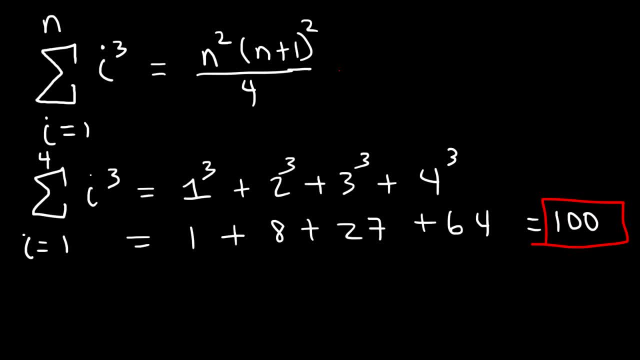 let's see if we can get the same answer using this formula. so I'm going to work it right here. so n is 4, that's going to be 4 squared, and 4 plus 1 is 5 divided by 4. so we can cancel a 4 leaving. 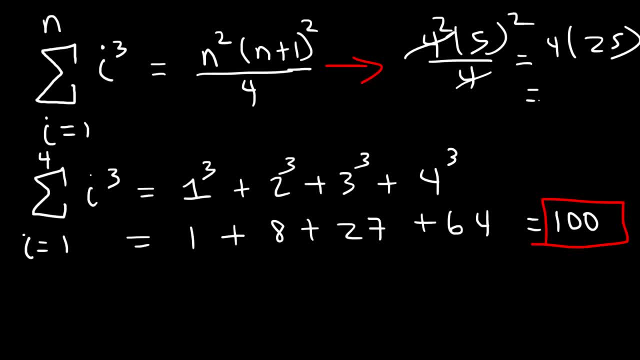 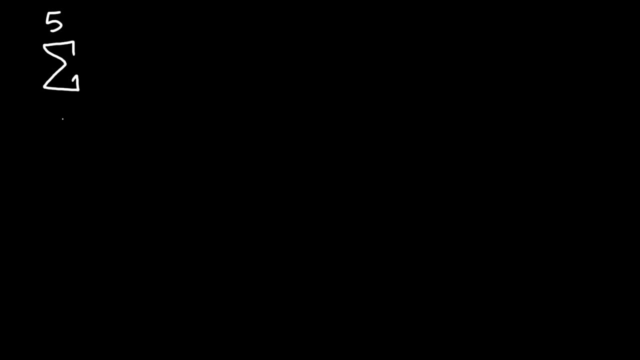 one: 4 on top 5 squared is 25, and 4 times 25 is 100. so this is the formula for I to the third. if you ever need to use it now, let's work on a few practice examples. so let's say: if we have I, 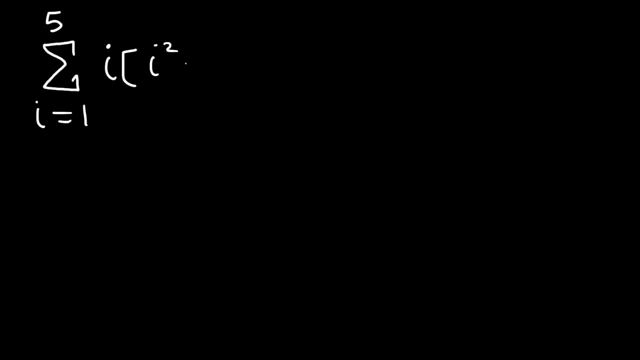 times I squared plus for I. go ahead and try this now. the first thing i recommend doing is to distribute the I i squared plus for i- so this is going to be i- to the third power of an eye times 4i. that's for i squared. and then we could. 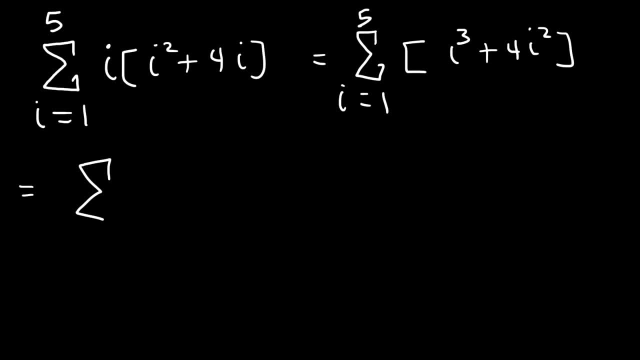 separate into two separate sides. So the first one is just i to the third power And for the second one it's going to be plus 4 times i squared. Now the formula for i to the third power is going to be n squared times n plus 1 squared. 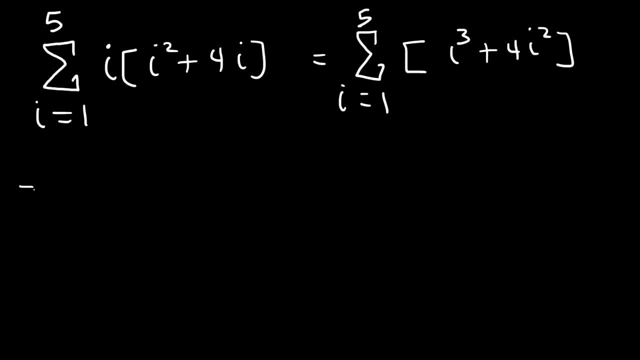 4i squared, and then we could separate it into two separate sums. so the first one is just i to the third power, and for the second one it's going to be plus 4 times i squared. now the formula for i to the third power is going to be n squared times n plus one squared over. 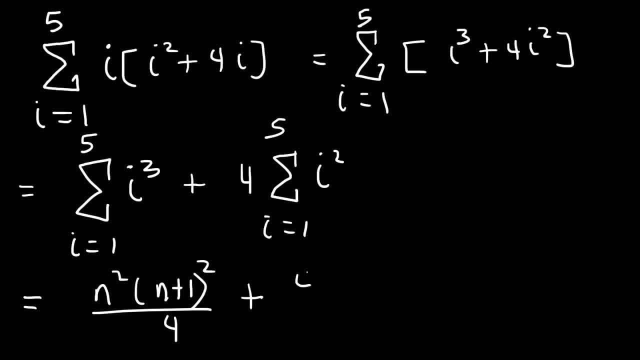 4, and then for the second one, it's going to be four times the formula for i squared, which is n and plus 1 times 2n plus 1 divided by 6. and keep in mind n is 5 based on what we see here. 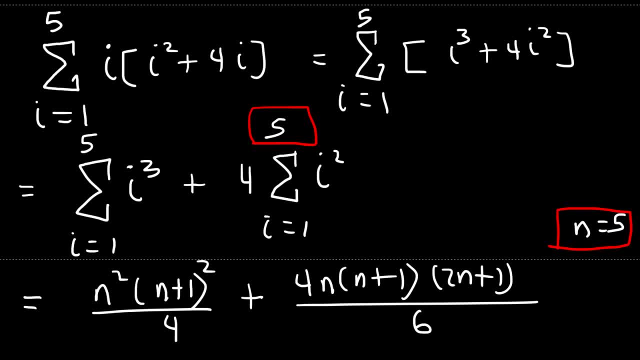 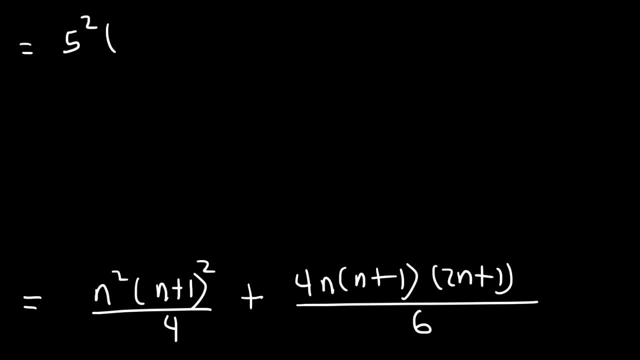 so let's plug in 5, this is going to be 5 squared, and then 5 plus 1 is 6. on the right we have 4 times 5, 5 plus 1 is 6,. 2 times 5 is 10 plus 1, that's 11 divided. 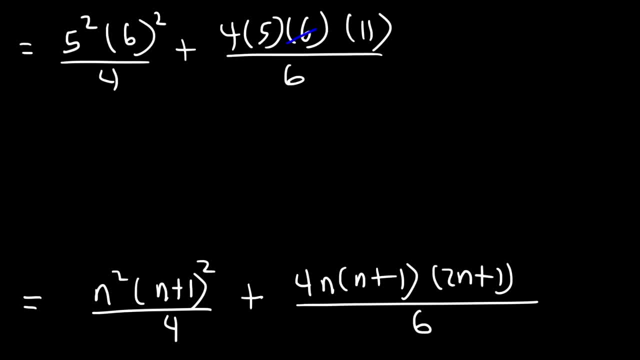 by 6, so at least we could cancel a 6 on the right side. now, 5 squared is 25, 6 times 6 is 36. on the right, 4 times 5 is 20. now, 36 divided by 4, that's a 9. and what's 20 times 11? so if you have 11 $20 bills, how much. 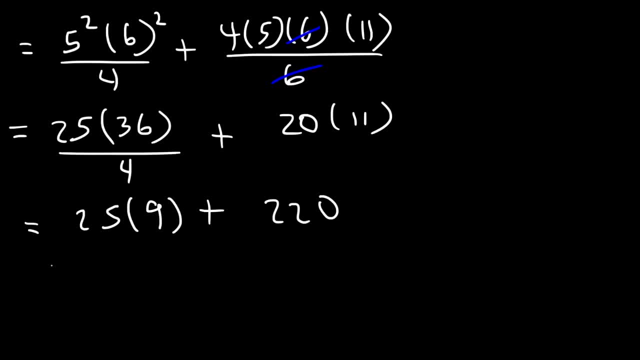 money do you have? that's going to be 220, and if you have 9 quarters, you have $2.25. so 25 times 9 is 225 plus 220, that's going to be 445, and that's the answer. now let's work on one last problem. 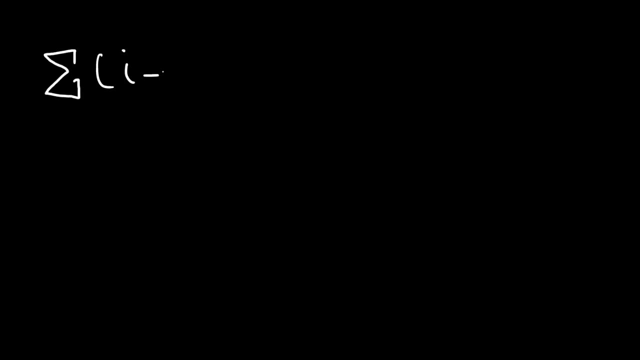 so let's say, if we have I minus 1 squared from 1 to 9, go ahead and evaluate it now. the first thing I would do is: for you, I minus 1 squared. so this is I minus 1, times I minus 1, and so I times I. that's. 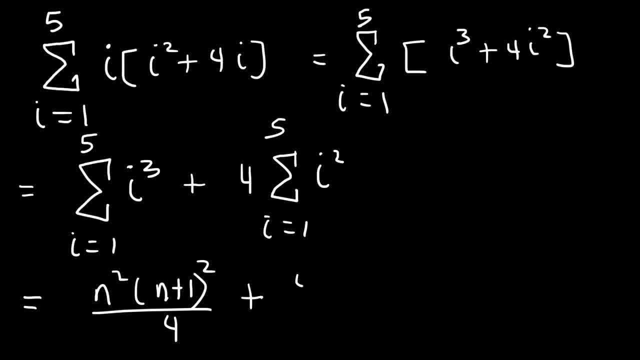 over 4.. And then for the second one, it's going to be 4 times the formula for i squared, which is n? n plus 1 times 2n plus 1 divided by 6.. And keep in mind, n is 5 based on what we see here. 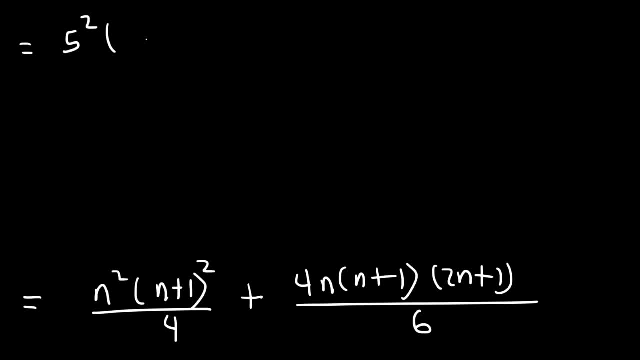 So let's plug in 5.. This is going to be 5 squared, and then 5 plus 1 is 6.. On the right we have 4 times 5, 5 plus 1 is 6,. 2 times 5 is 10 plus 1, that's 11, divided. 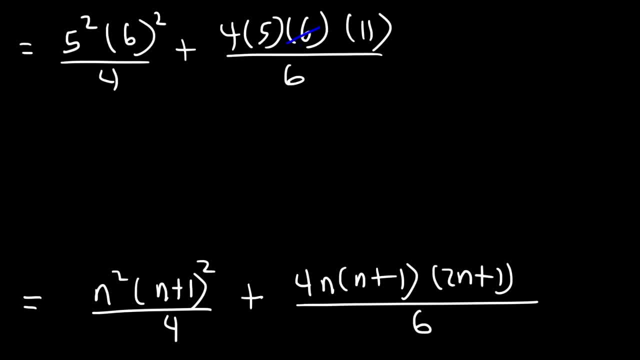 by 6.. So at least we could cancel a 6 on the right side. Now, 5 squared is 25, 6 times 6 is 36.. On the right: 4 times 5 is 36.. On the right: 4 times 5 is 36.. 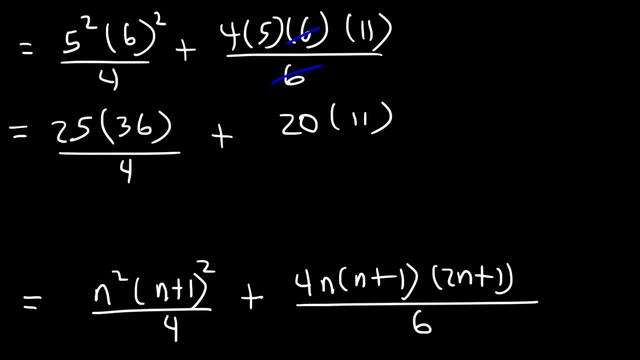 On the left. 4 times 5 is 20.. Now 36 divided by 4, that's a 9.. And what's 20 times 11?? So if you have 11 $20 bills, how much money do you have? 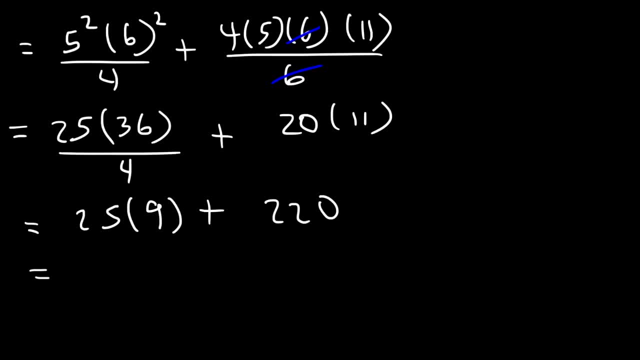 That's going to be 220. And if you have 9 quarters, you have $2.25.. So 25 times 9 is 225.. Plus 220, that's going to be 445.. And that's the answer. 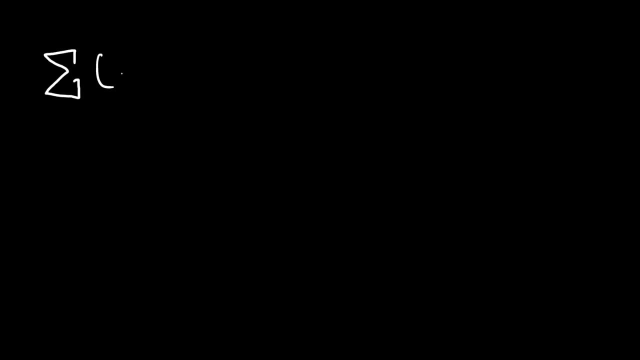 Now let's work on one last problem. Let's say we have i minus 1 squared from 1 to 9.. Go ahead and evaluate it Now. the first thing we would do is FOIL i minus 1 squared. So this is i minus 1 times i minus 1.. 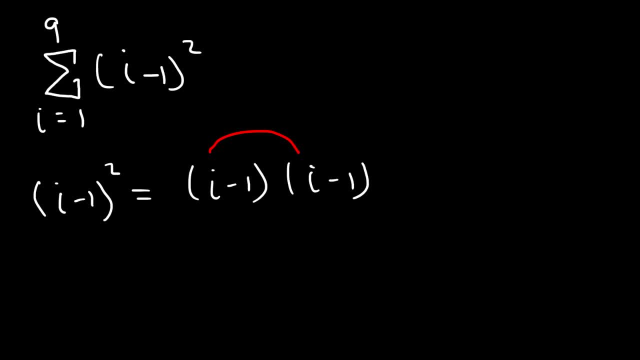 I'm going to count how I do myuire down Now. I'm just going to follow the equation. I'll write one x yuan one and I'll put one side down. So 1 divided by 1 times 1.. I, that's going to be I squared, and then we have I times negative 1, so that's. 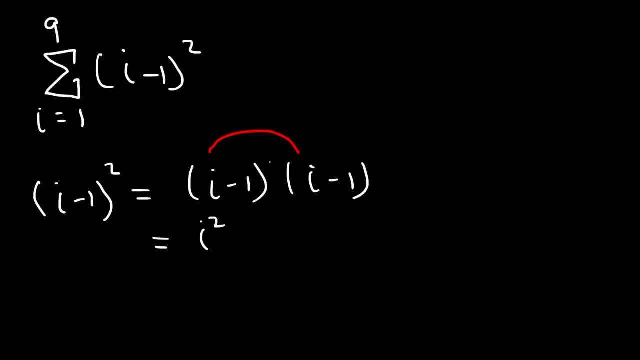 going to be I squared. and then we have I times negative 1, so that's negative I. negative 1 times I is also negative I. and then the last one is negative 1 times negative 1, which is positive 1. so now let's combine like terms, so this: 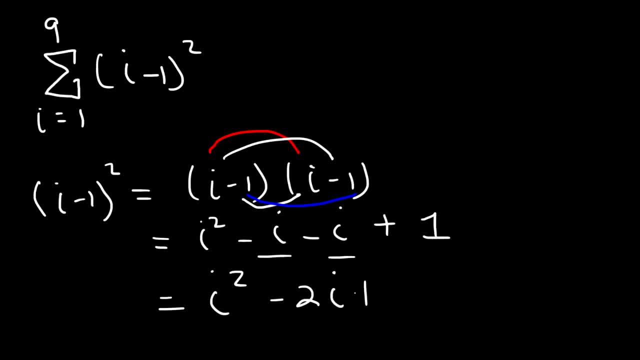 becomes: i squared minus 2, i plus one. so we can rewrite the problem like this: now let's separate it into three separate sums. so we have I square from 1 to 9, and then minus 2 times the sum of i from 1 to 9, and then we have a constant. 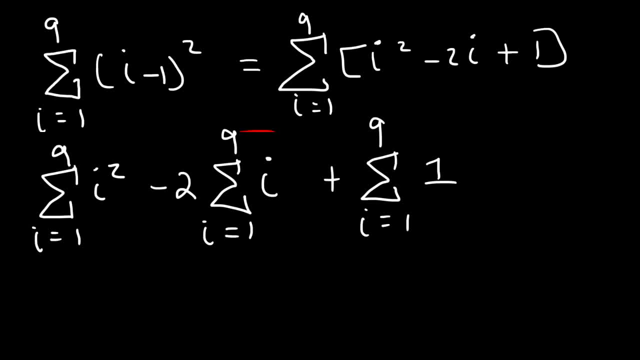 So now let's employ the appropriate formulas. So for i, squared, it's going to be n times n plus 1 times 2n plus 1 divided by 6, and then minus 2 times the formula for i, which is n, n plus 1 divided by 2.. 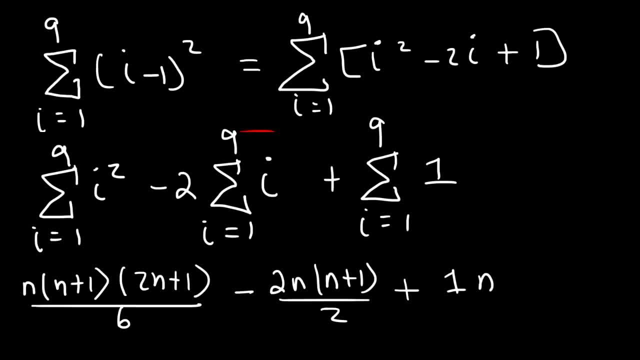 And for the constant, it's just going to be the constant times n, And keep in mind n is equal To 9 for this problem. So on the left it's going to be 9, and then 9 plus 1 is 10,, 2 times 9,, which is 18 plus 1, that's 19.. 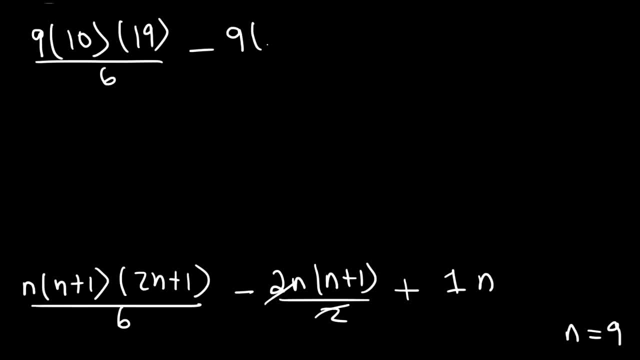 Here we could cancel the twos, And so it's going to be 9 times 9 plus 1, which is 10, and then plus n, so that's 9.. Now, 9 times 10 is 90.. And on the right we also have another 9 times 10, which is 90 as well. 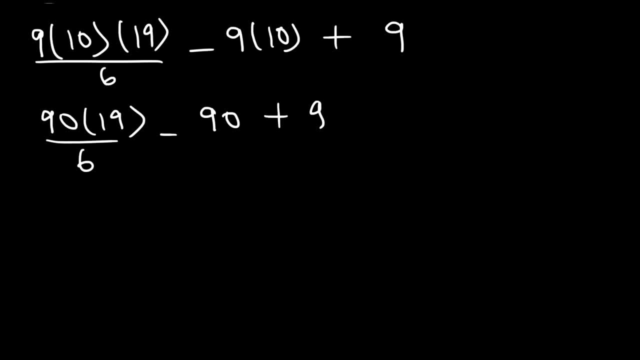 90 divided by 6 is 15.. So we have 15 times 19, and 19 is just 20 minus 1.. Negative 90 plus 9, or 9 minus 90,, that's negative 81.. Now, 15 times 20 is 300. 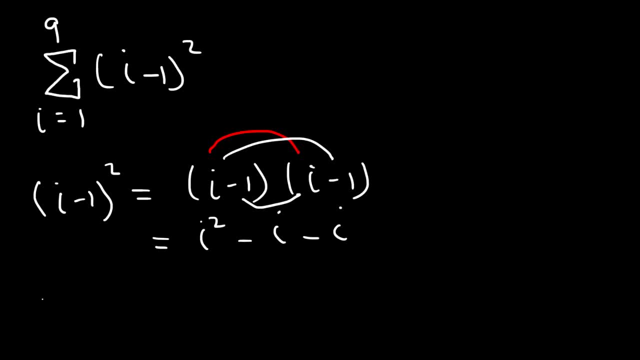 negative I negative 1 times I is also negative I. and then the last one is negative 1 times negative 1, which is positive 1. so now let's combine like terms so this becomes I squared minus 2i plus 1, so we can rewrite the problem. 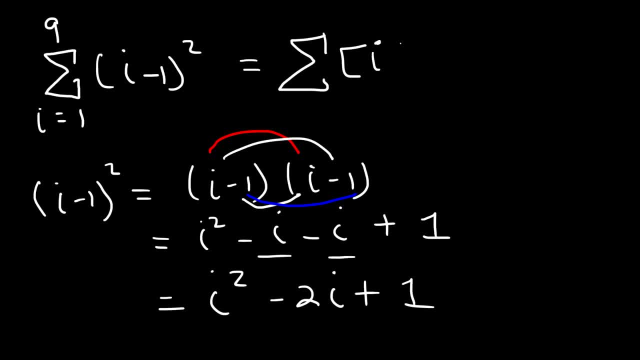 like this: now let's separate it into three separate sums. so we have I squared from 1 to 9, and then minus 2 times the sum forward of I from 1 to 9, and then we have a constant. so now let's deploy the. 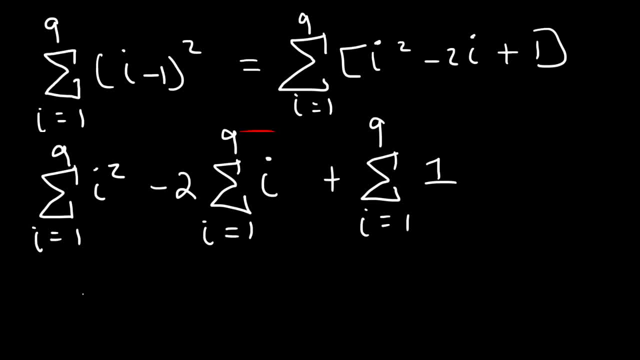 appropriate formulas. so for I, squared is going to be n times plus 1 times 2 plus 1 divided by 6, and then minus 2 times the formula for i, which is n n plus 1, divided by 2.. And for the constant, it's just going to be the constant times n. 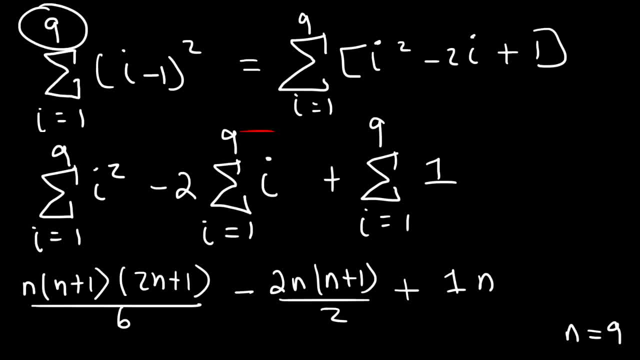 And keep in mind n is equal to 9 for this problem. So on the left it's going to be 9, and then 9 plus 1 is 10.. 2 times 9,, which is 18 plus 1,, that's 19.. 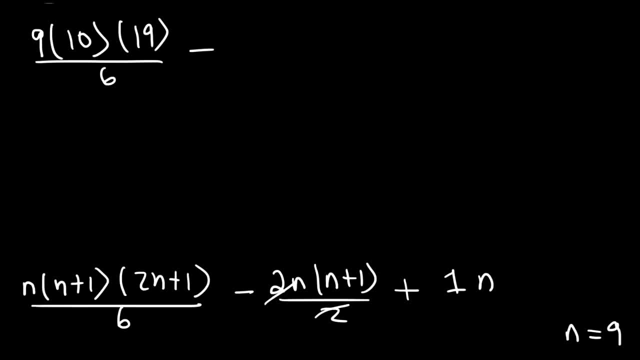 Here we could cancel the 2s, And so it's going to be 9 times 9 plus 1,, which is 10.. And then plus n, so that's 9.. Now, 9 times 10 is 90.. 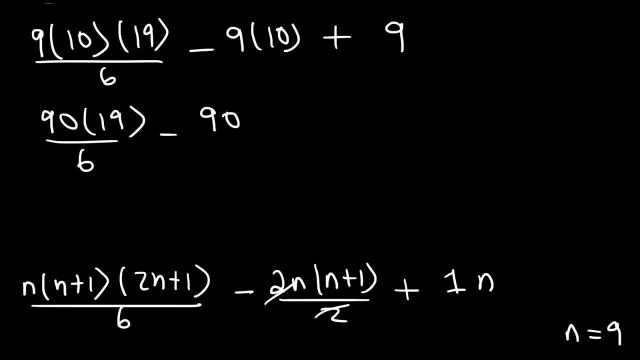 And on the right we also have another 9 times 10, which is 90 as well. 90 divided by 6 is 15.. So we have 15 times 90. And 19 is just 20 minus 1.. 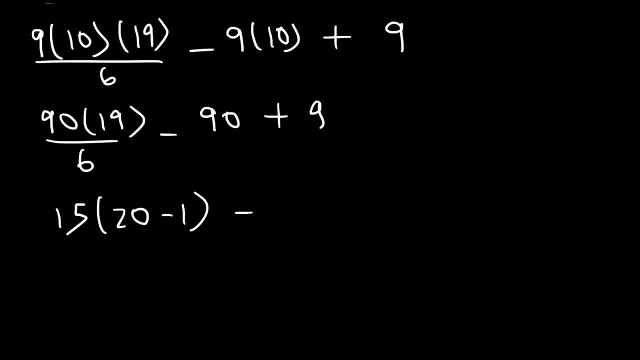 Negative: 90 plus 9, or 9 minus 90,, that's negative 81.. Now 15 times 20 is 300.. And 15 times 1 is 15.. So 15 times 19 is really 285..